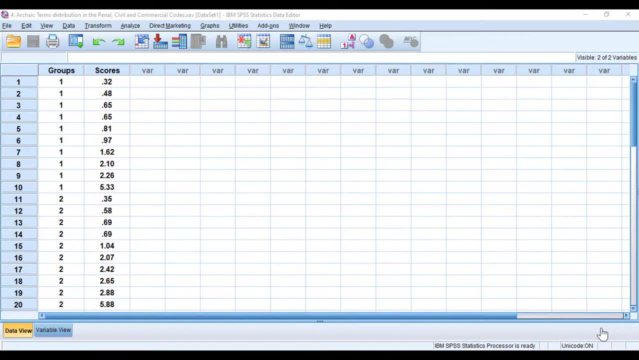 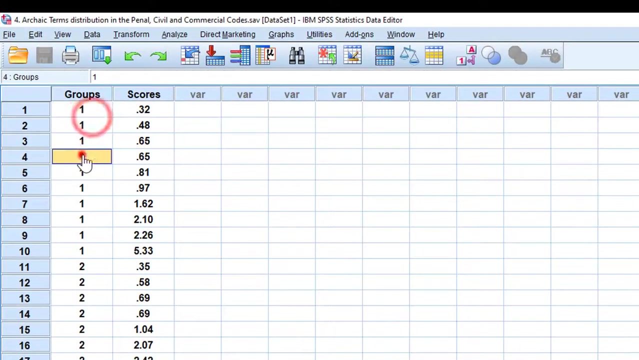 Hello everyone, I hope you are doing great. Today. I am going to show you how to run a cross-call wallace test using SPSS version 23,. interpret the results as well as write them in the report. So we have our data entered in this way. So we have three groups: categorical groups. 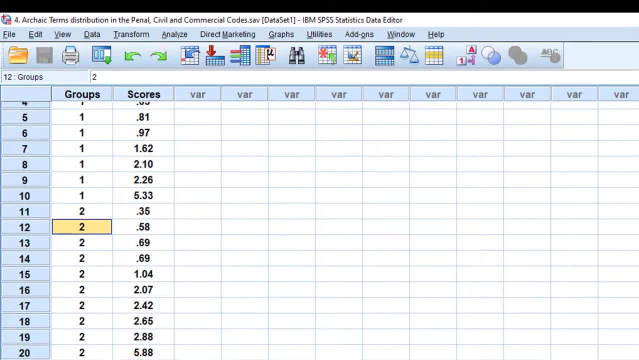 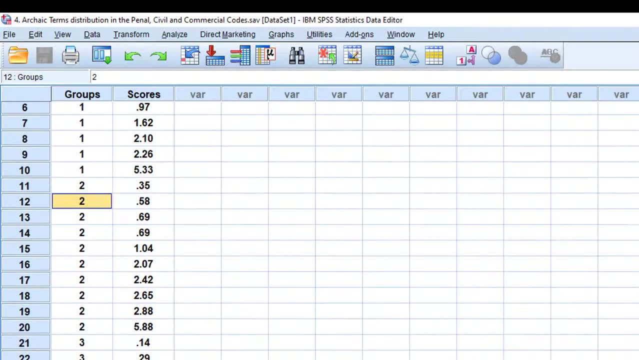 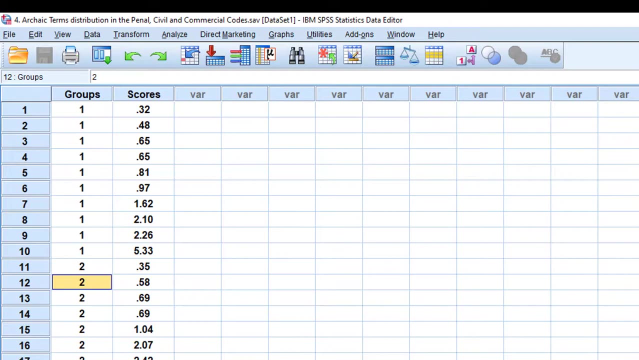 and we have their corresponding scores, as you can see, and we want to see whether or not there is any difference or statistically significant difference between or the the medians of these groups. So we try to to use the one-way ANOVA test, but there is an assumption of 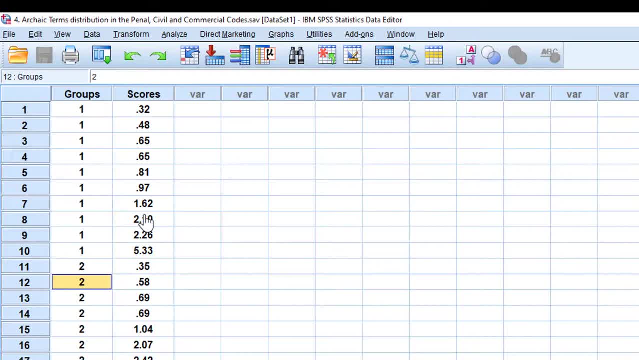 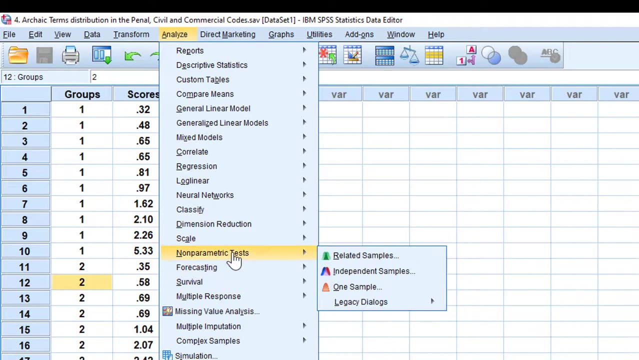 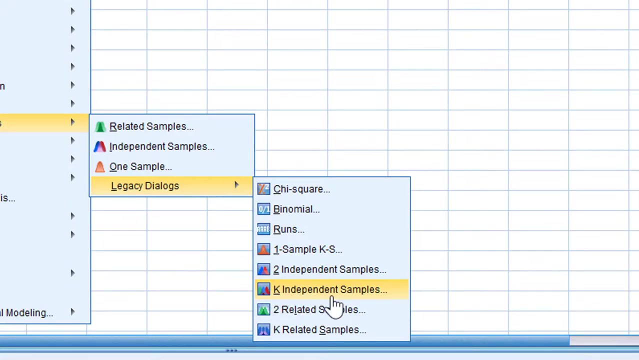 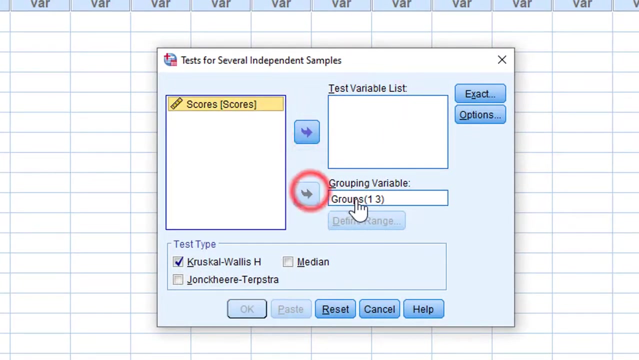 a normality that is violated. therefore, we resorted to the cross-call wallace test. So here we go to analyze, and then we go to non-parametric tests, and then we choose legacy dialogs and then we click on key independent samples Once clicked. so I'm going to reset this to show you how I did it. so we move, I move the. 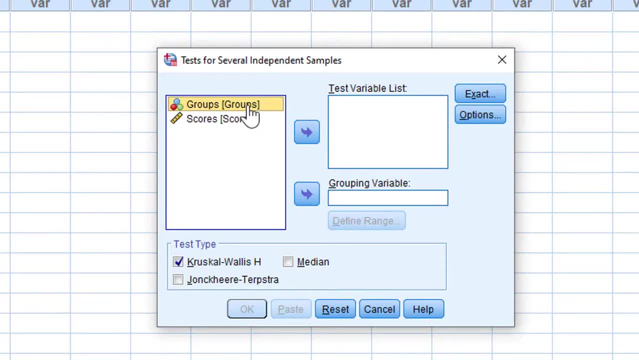 categorical variable, that is, groups, in this case to the grouping variable and the scores, which is, by the way, continuous variable, ratio variable to test list. Then I check cross-call wallace H and before checking that and moving to the analysis, I'm going to define groups. so I click on. 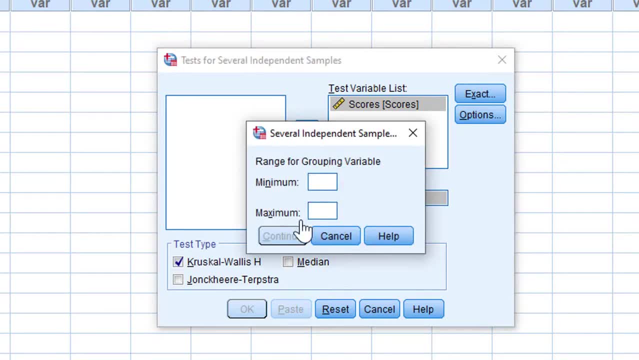 the groups and click define range, So the range between minimum and maximum. so I coded the variables from 1 to 2, if you go to 3, so I'm going to put the minimum 1 and the maximum 3 and click continue. 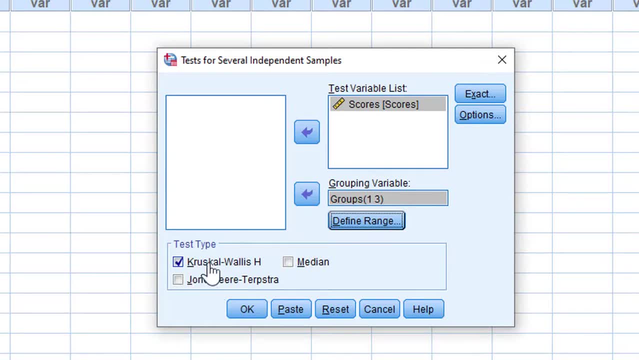 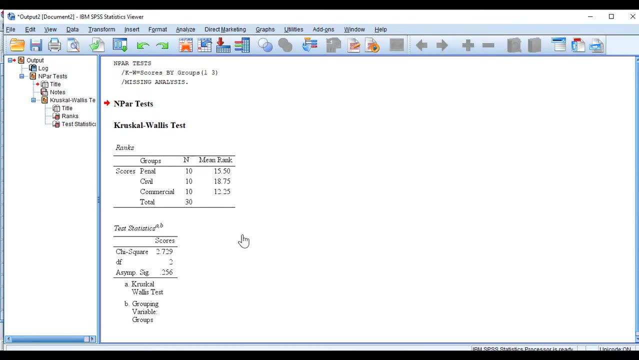 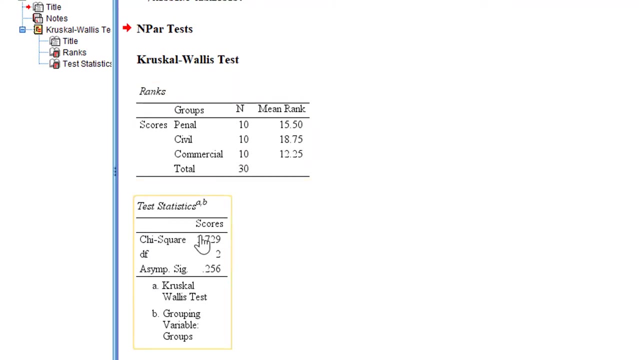 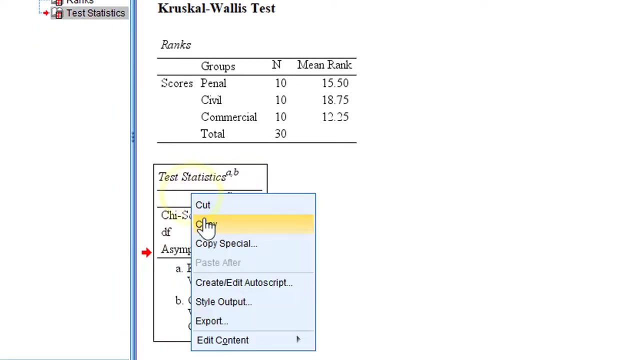 After that. so we already checked the cross-call wallace H test. so I click OK and here is the output. So now I should interpret this output and write it in the report. So here I use this table of test statistics, so I'm going to copy and paste it to my report and then explain. 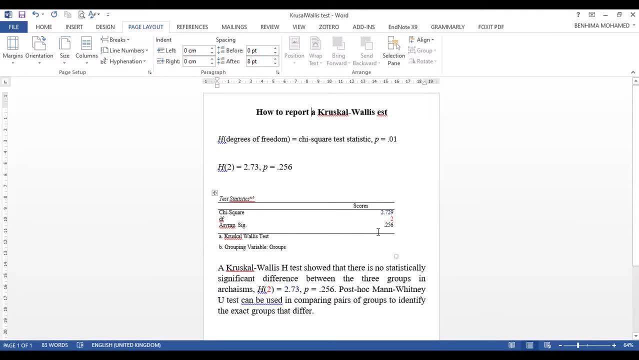 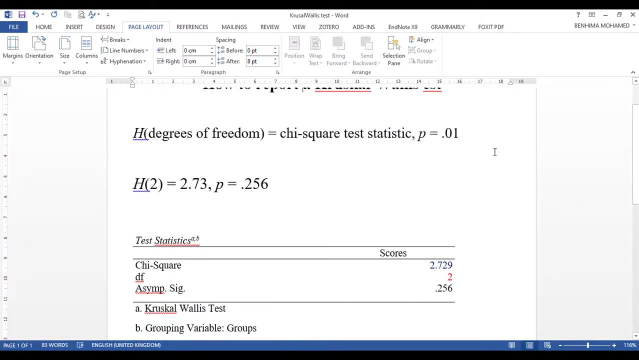 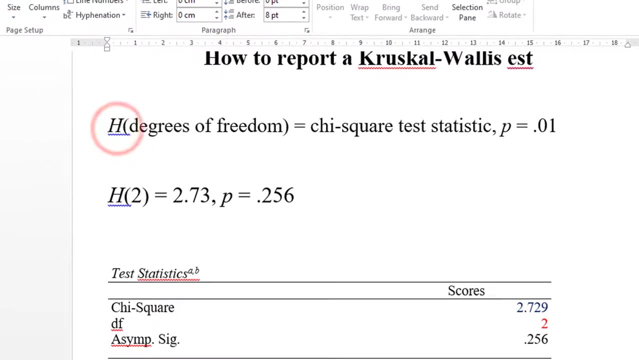 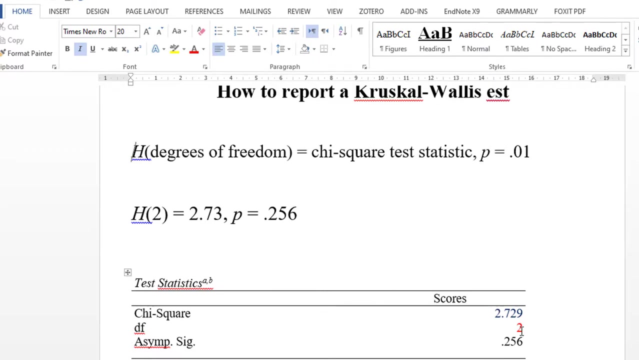 So this is the table that I took from spaces and this is how the result of cross-call wallace test should be written. So I write H in italics, if you are writing in APA style, and then put the values of the degrees of freedom, which are in this case two DF, then put equal values of Jeremy ´ônd this値, although N is EES. Which are in this case to DF. Then put equal to D hundred, D hundred call all the way up to then D x. We of course will use superior set very quickly, But if you wanna write this in th las, value 1.. value 1.. So this is the table that I took from space S and this is how the results of cross-call wallace test should be written. And this is how the result of cross-call wallace test should be written. So I add: 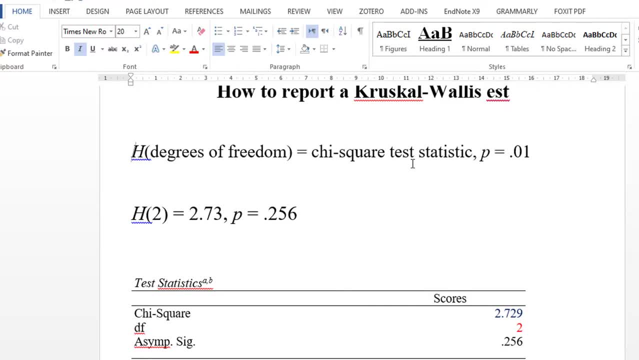 equal chi-square test statistic. so then I'm going to choose to move to this chi-square test statistic and see its value. so I'm going to put this value here and then put the value like this in italics: equal and write the significance. here we have a simp 662, 256 out of 1000 or 25 percent. so anyway, this value as: 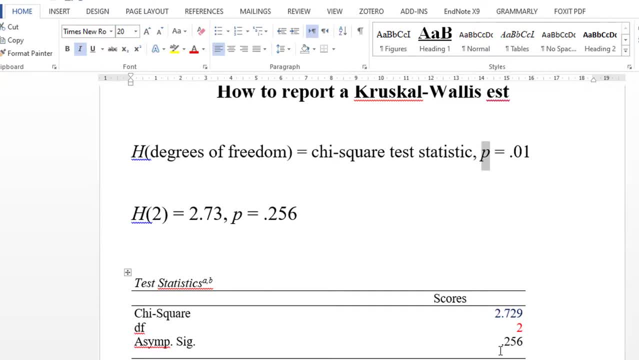 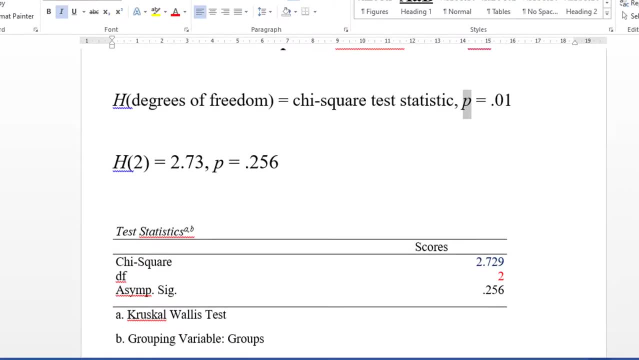 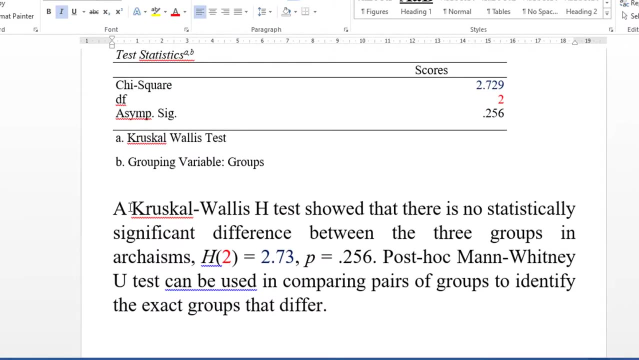 you can see, is greater than 0.05. therefore we fail to reject the null hypothesis that states that there is no statistically significant difference in the middle of these groups. so I can say that cross-color is each test so that there is no statistically significant difference between the three groups in our case. for